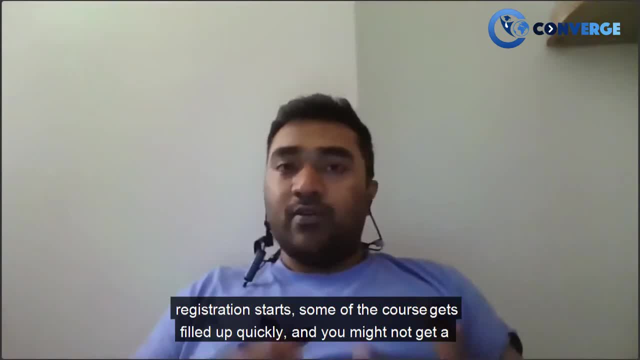 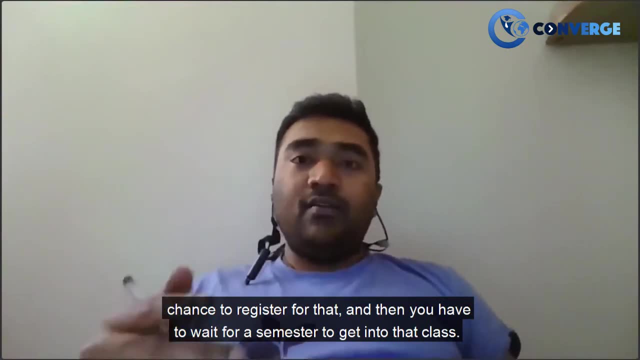 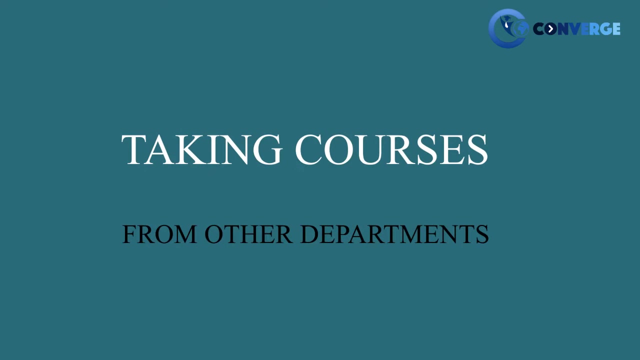 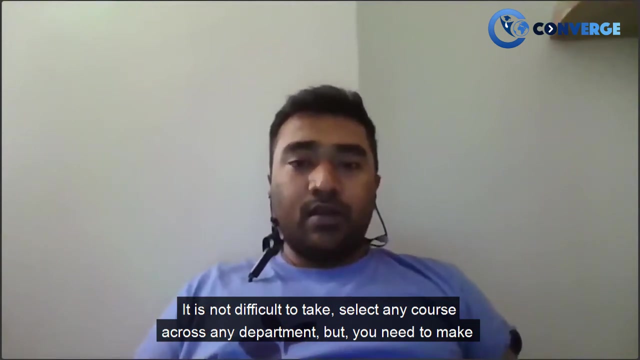 As soon as the course registration starts, some of the course gets filled up quickly and you might not get a chance to register for that, And then you have to wait for a semester to get into that class. It is not difficult to select any course across any department, but you need to make sure that you possess 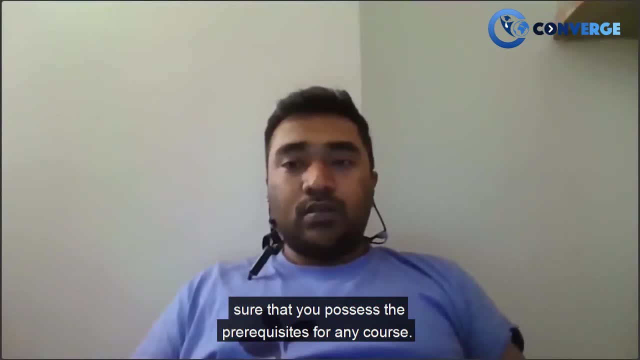 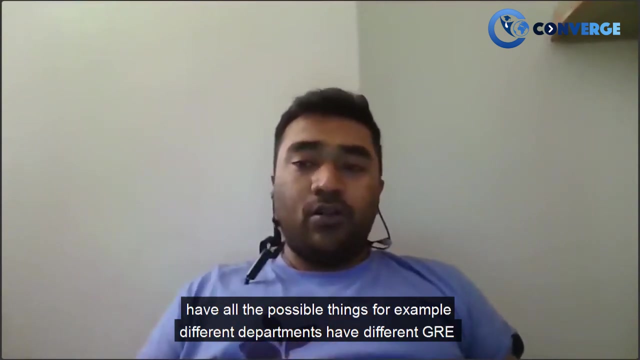 the prerequisites for any course. It is definitely possible to switch into any department if you fit into the criteria, If you have all the possible things. for example, different department has different GRE cut-offs. different department has different TOEFL cut-offs. 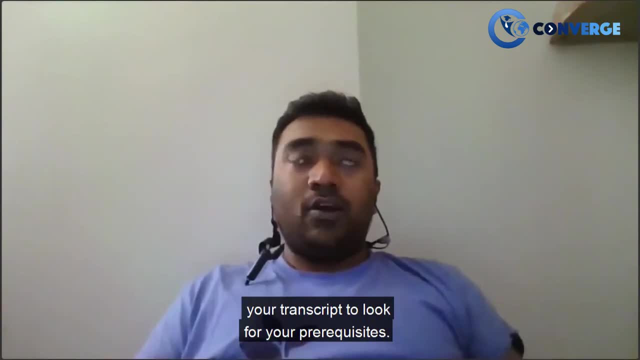 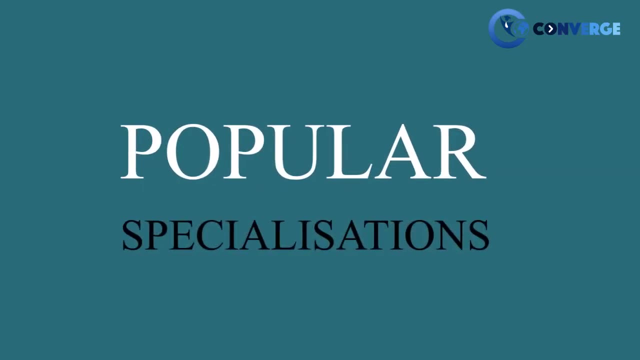 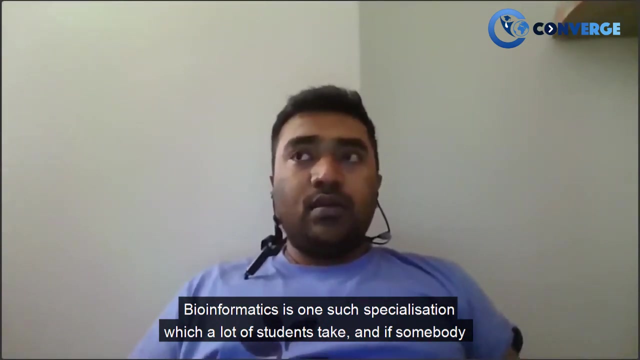 Different department might require your transcript to look for your prerequisite. Bioinformatics is one such specialization which a lot of students take, And if somebody wants to be more specialized into something then they eventually go for a PhD. It is more towards the theory part. 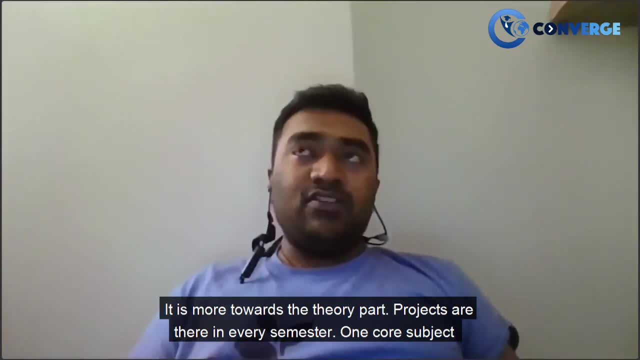 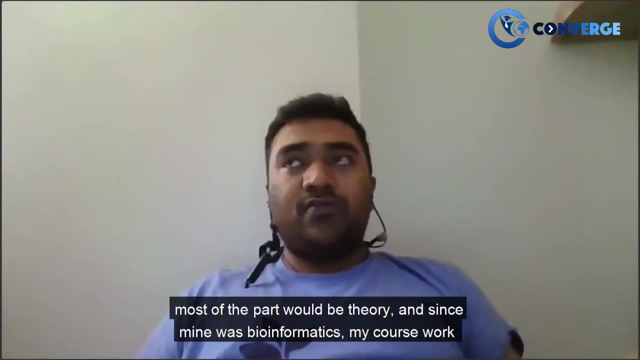 Projects are there in every semester. One core subject would have a project that you need to submit eventually at the end of the semester, But most of the part would be theory, And since mine was bioinformatics, my coursework included a lot of programming too. 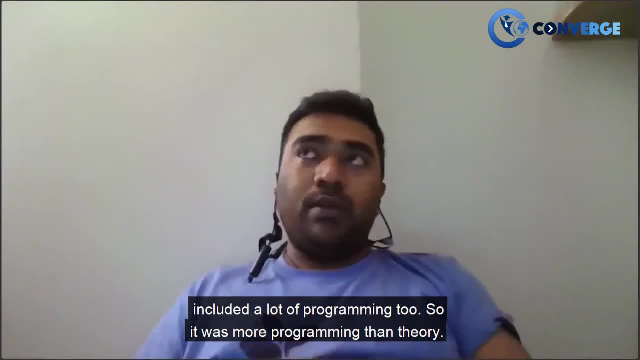 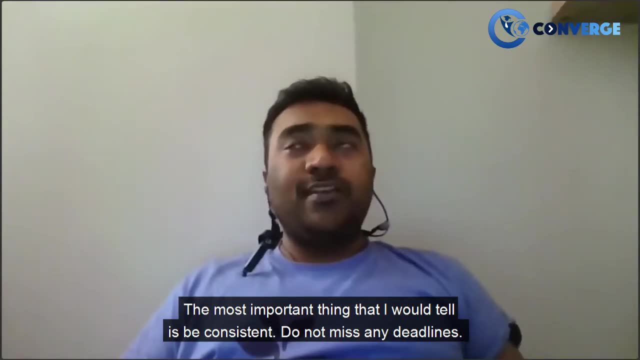 So it was more programming than theory. The most important thing that I would tell is be consistent. Do not miss any deadline. Submit all the assignments. That's the most important thing, Even if you might have not completed the assignment. submitting is more important than not submitting. 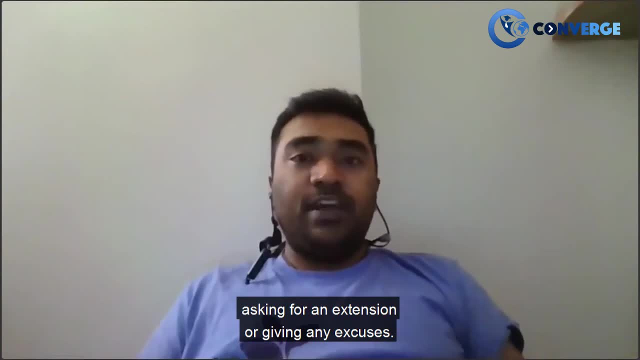 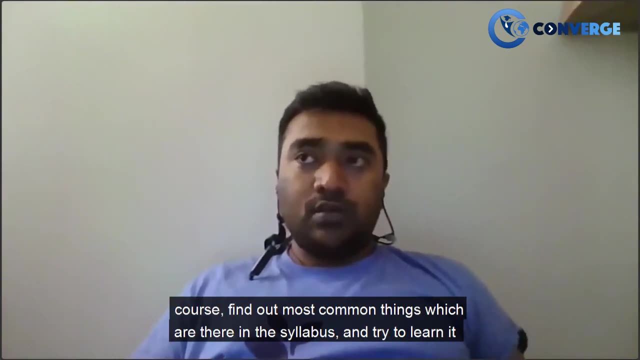 and then asking for an extension or giving any excuse. Whichever course they are taking, Whichever course they are going for in masters, Just look at the syllabus, Look at the course. Find out most common things which are there in the syllabus.